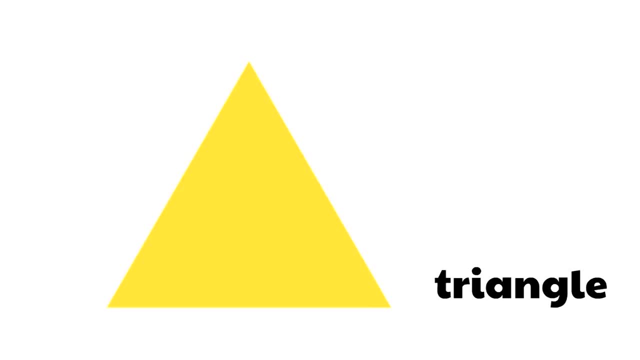 So let's count the sides together: One, Two, Three. This shape has a triangle. This shape has three sides. A triangle has three sides. Not all triangles look the exact same. Look at this triangle. We know that this is a triangle because of its sides. 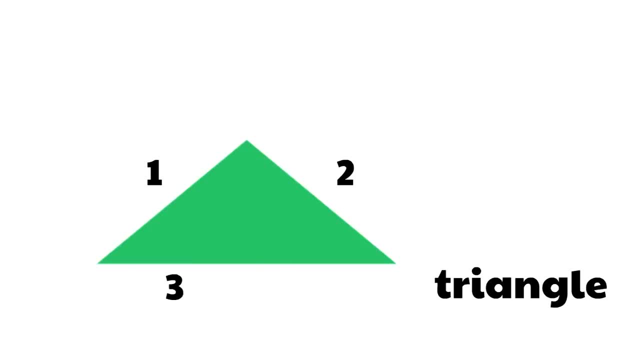 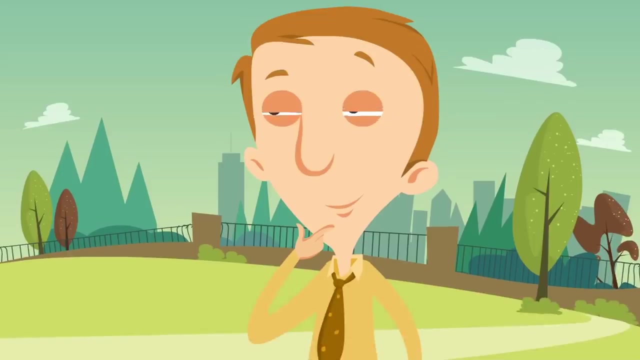 Let's count them together: One, Two, Three. There are three sides. Every triangle has three sides. It just looks more squished than the other triangle, But it's still a triangle. Now here is something very interesting, very interesting. 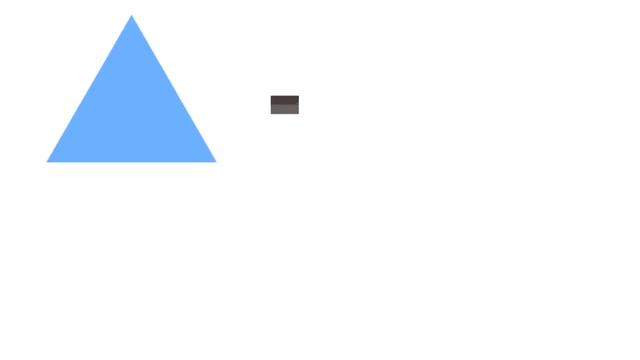 Let's say we took the triangle and we stretched it out. It's still a triangle, right? But if you did the same thing to the circle, if you stretched out that circle, it actually becomes a different shape, A shape called what? 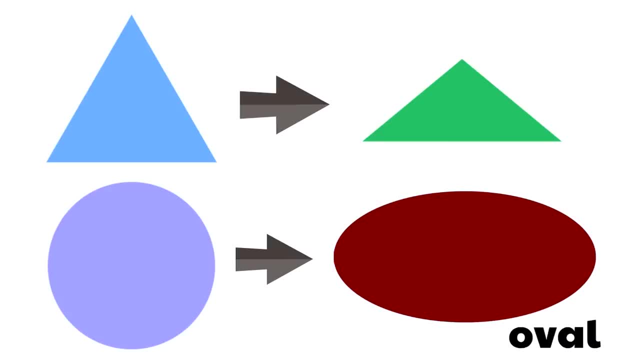 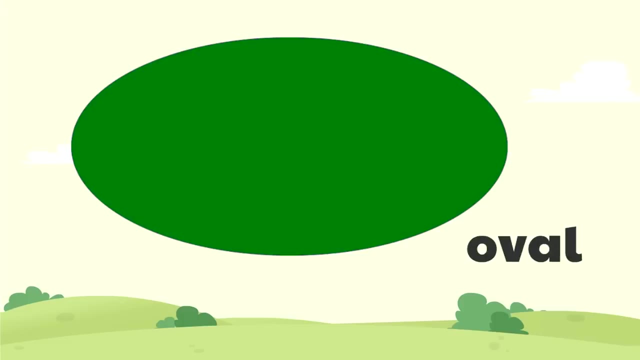 Yeah, an oval, An oval, An oval. When you stretch out a circle it becomes an oval, And that's our third shape. Here it is again An oval, An oval. An oval is a stretched out circle, basically right. 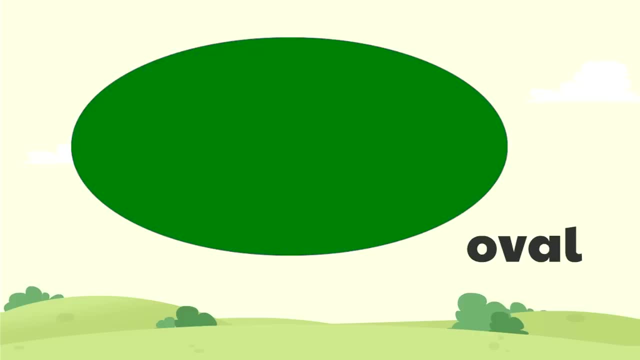 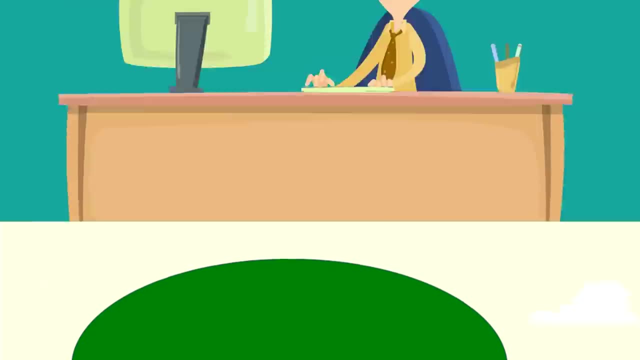 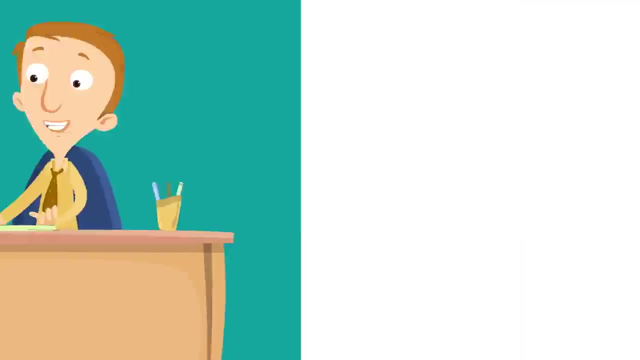 An oval. You've seen these around right. Can you say that with us? Oval, Oval. Good, Let's look through these three shapes again just to make sure we really know them. What is this shape? Yeah, a triangle. 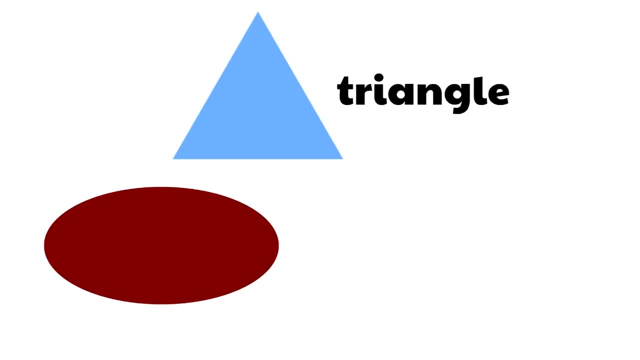 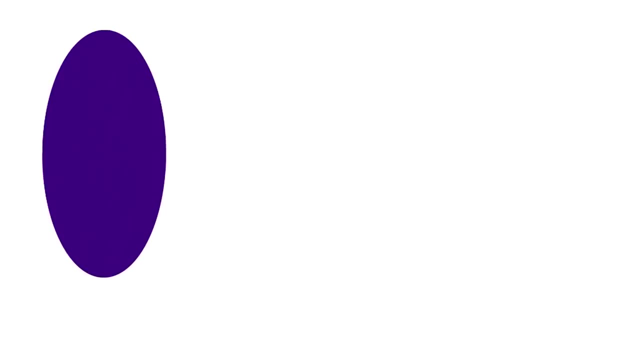 What's this shape, Do you know? Yeah, it's an oval. What's this shape? Yeah, a circle. Okay, what is this shape? Yeah, it's an oval. What is this shape? Uh-huh, It's a triangle. 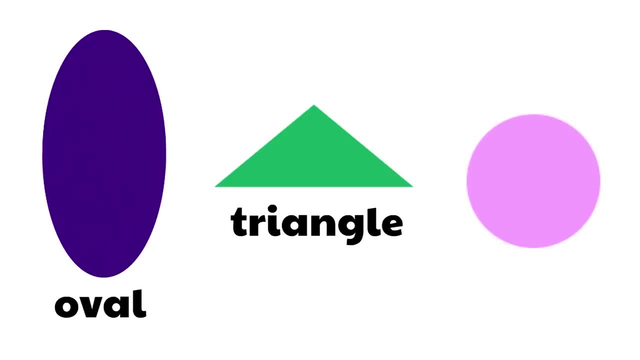 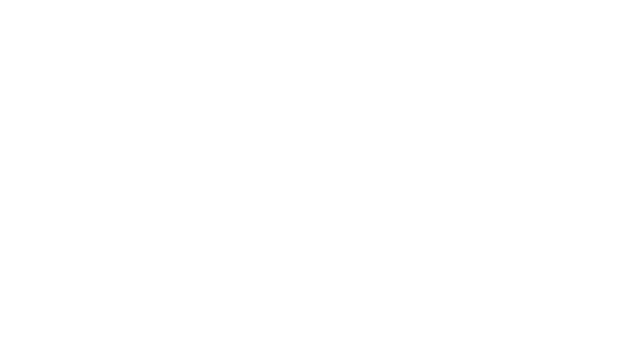 What is this shape? Yeah, a circle. Now we're going to get help from our friend Clarence, who's going to show us the next four shapes. okay, The next four shapes all have one thing in common: They have four sides. 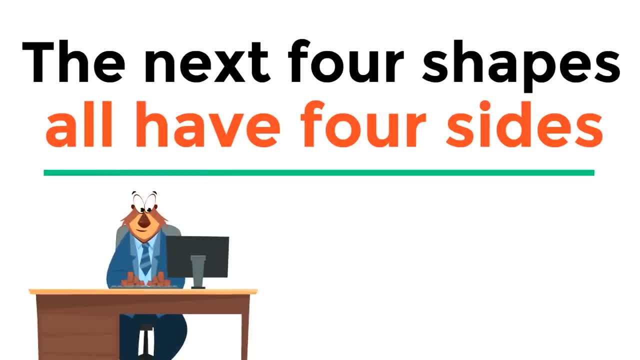 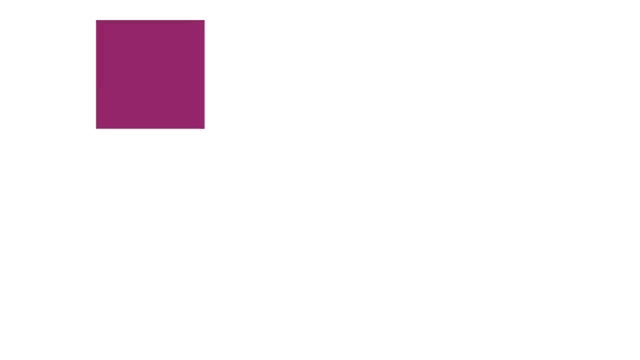 Four shapes that have four sides. So let's meet these shapes. The first one is this shape. This shape is a square, A square, A very common, very popular shape. The next shape is this shape: What is this shape? What is this shape? 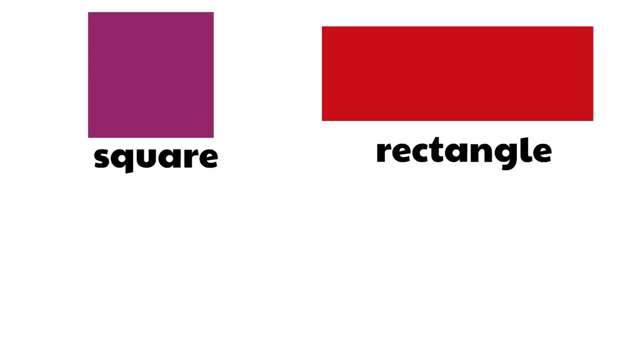 Do you already know? Yeah, a rectangle, A rectangle. The next shape is not as popular and you might not be familiar with it. This shape is a trapezoid. Oh, that's a fun word to say. Can you say trapezoid? 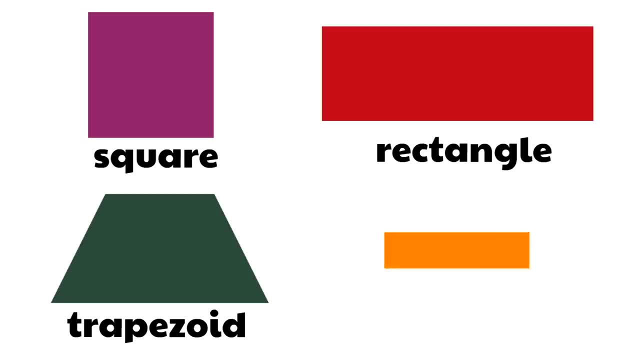 Wow, trapezoid. And the final shape is this one, which is a parallelogram: Wow, parallelogram. Yeah, a trapezoid, Yeah, a trapezoid. First, let's look closer at the square, okay. 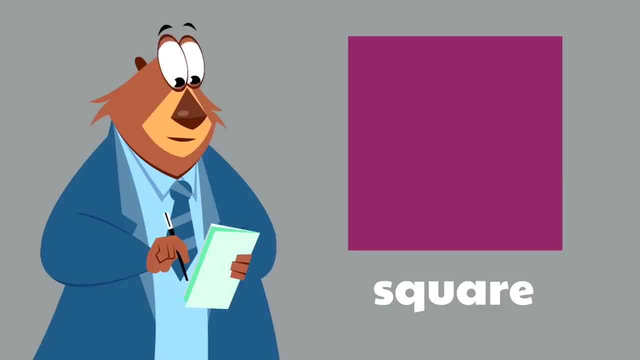 The square has four sides, of course, but all four of the sides are the same length. Okay, so it looks like a perfect box, doesn't it A square? A square has four sides that are all the same length. Next, we're going to take a closer look at the rectangle. 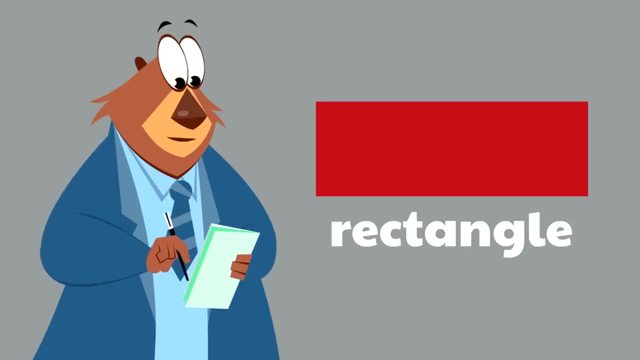 Yeah, rectangles are pretty cool. They are usually drawn like stretched-out squares, aren't they? It almost looks like a square that's been stretched out, But a rectangle is any shape that has four sides and has four corners that look like these. 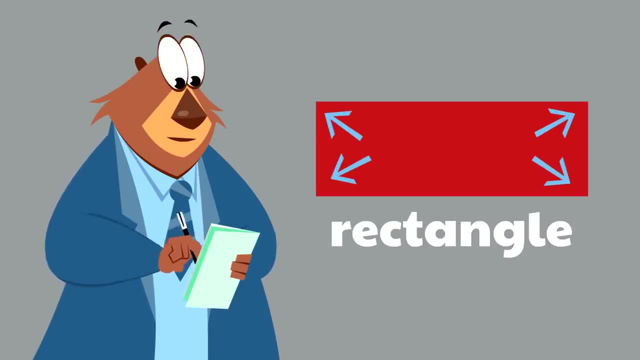 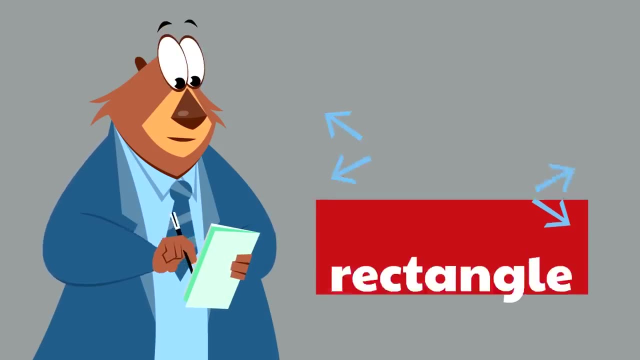 And they're usually drawn like this, so they can be drawn differently. They're usually drawn like a stretched-out square. They're usually drawn like a stretched-out square. They're usually drawn like a stretched-out square. Next, we are going to take a closer look at the trapezoid. 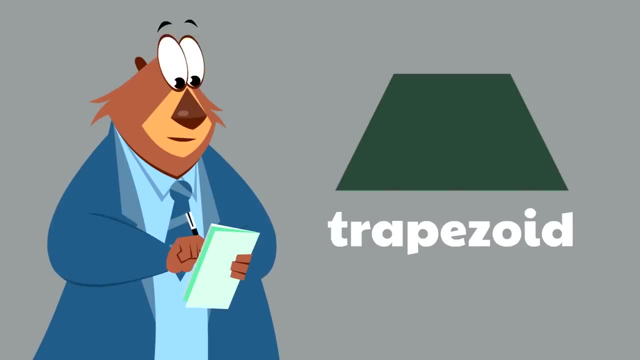 What a cool shape name trapezoid. Two of the sides are parallel to one another and the other two sides are not. That's what makes a trapezoid a trapezoid. You might be wondering: what does parallel mean? 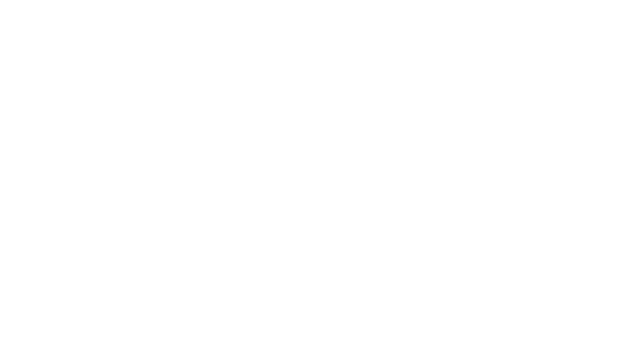 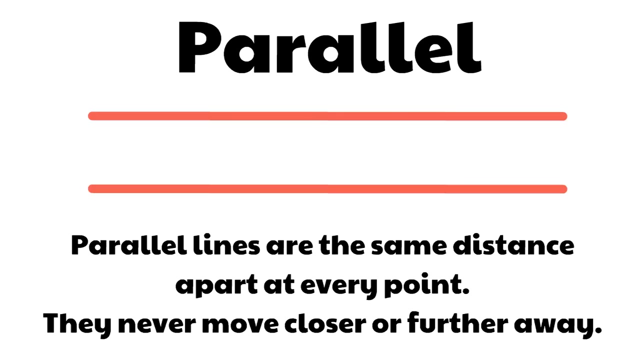 Well, let's show you. We'll show you with these lines. These lines are parallel to one another. Parallel lines are the same distance apart at every point. They never move closer or further away. Let's look at our trapezoid again. 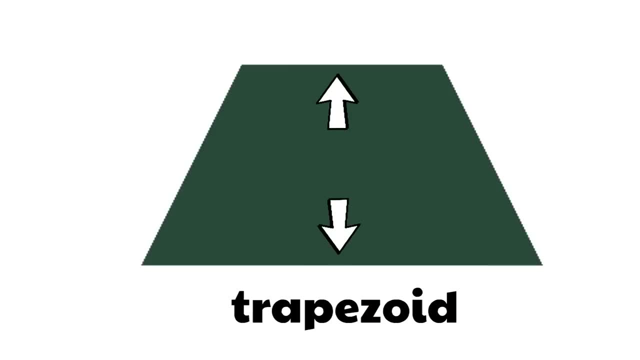 The top side and the bottom side. those are parallel to one another because at every point they're the same distance from each other, aren't they? But what makes a trapezoid so unique is: look at these two sides. These two sides are not parallel to one another. 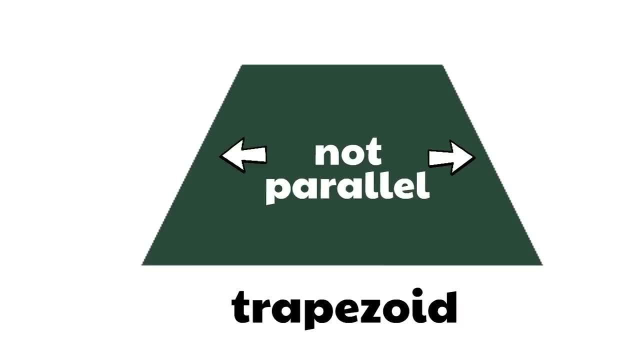 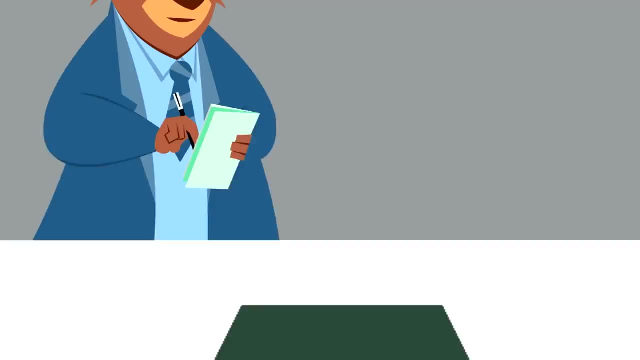 They're actually moving apart as you move down the shape, don't they? Those sides are actually moving away from one another. They are not parallel to one another. That's what makes this shape a trapezoid. Okay, Clarence, we hope you're ready. 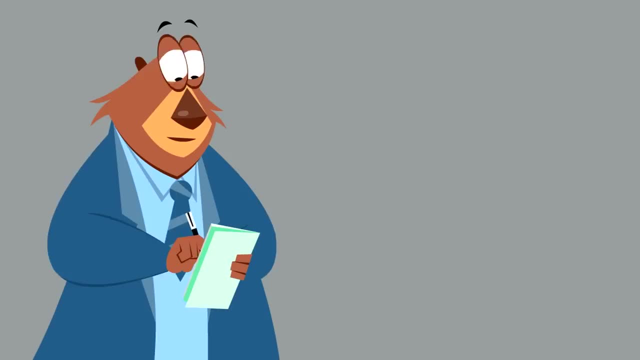 The last four-sided shape that we're going to be looking closer at is the parallelogram And, as the name might suggest, it's named after the fact that the opposite sides of the parallelogram are always parallel to one another. That's what makes a parallelogram. 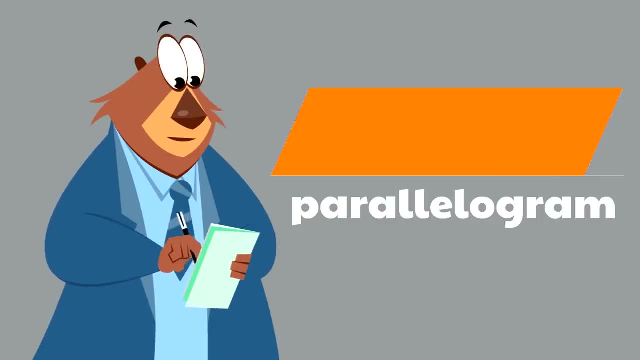 a parallelogram. A parallelogram can be drawn in many different ways, but this is the most popular way to draw a parallelogram: To draw it almost like a rectangle. that is having the wind blow really fast towards it so it's almost bending backwards. 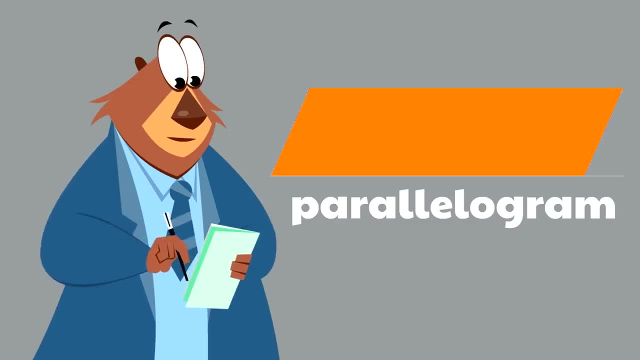 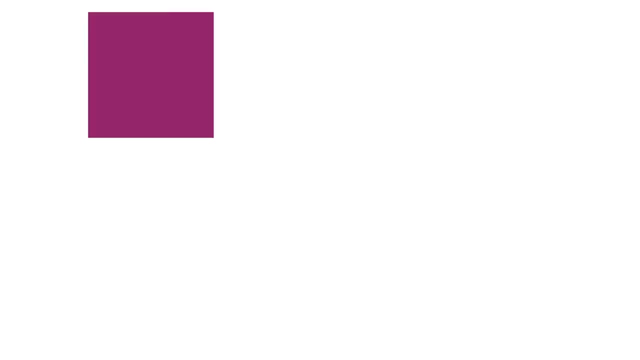 It's almost looking like a slanted rectangle. That is the way that a parallelogram is usually drawn. Okay, so what's this shape, Do you remember? Yeah, a square. And what about this shape? Uh-huh, a rectangle. 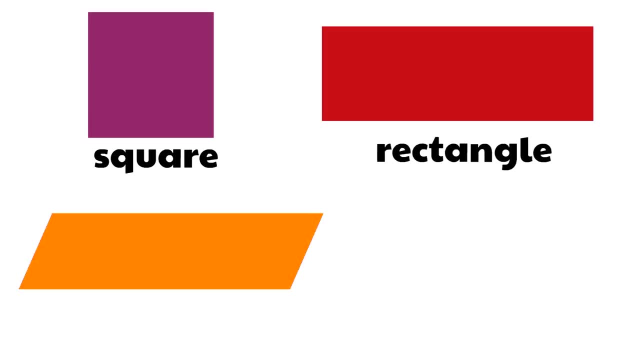 What about this shape? Uh-huh, it's a parallelogram. And what about this shape? What's this? Uh-huh, a trapezoid. Hey, Clarence, thanks for helping us. We'll see you next time. 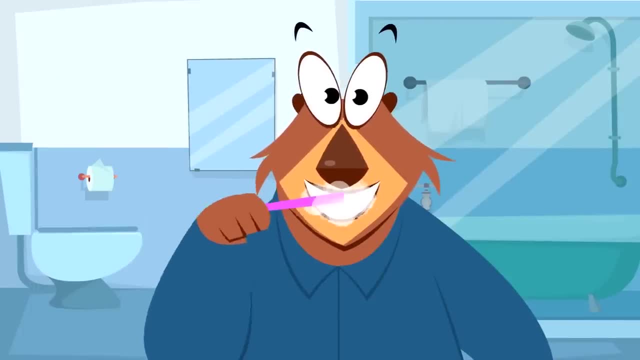 Clarence, thanks for helping us. Oh, are you brushing your teeth? Okay, well, good for you. That's awesome. Thanks for helping And, wow, it's important to brush your teeth. This is great. I didn't know bears brushed their teeth. 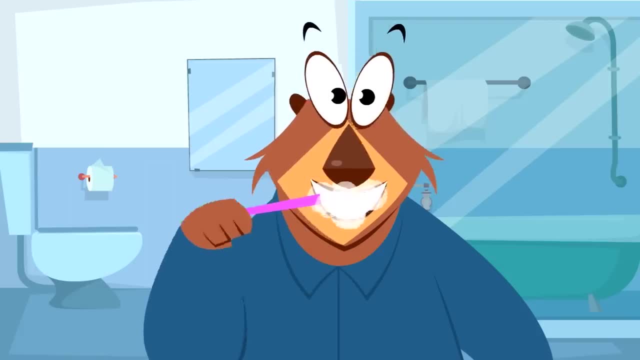 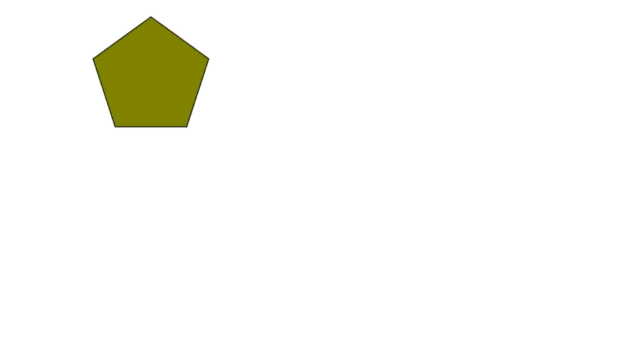 but that's phenomenal. That's great. All right, we've got more shapes to cover here. We've got to go. Sorry, Clarence, We're going to leave your bathroom now. We only have three more shapes to show you. The first is the pentagon. 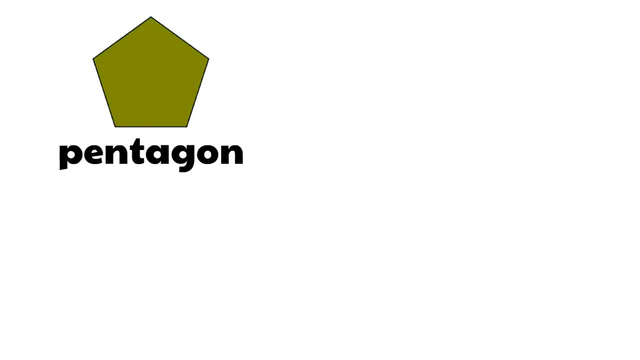 The pentagon has five sides. Next is the hexagon. The hexagon has how many sides? Uh-huh, six, Six sides. A hexagon has six sides, And the final shape we're showing you today is the octagon. 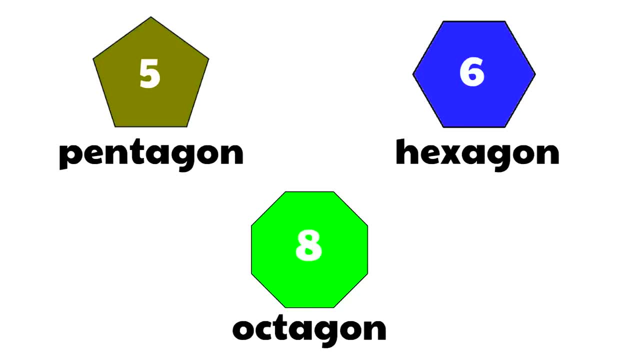 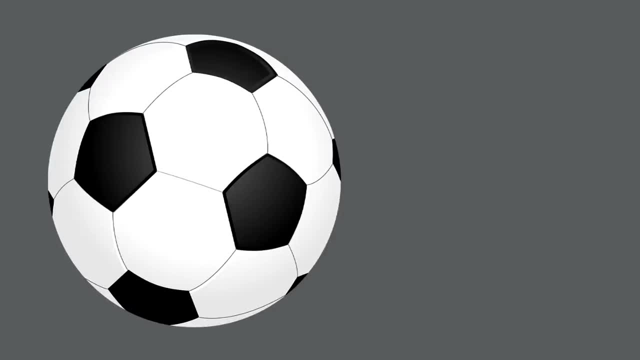 The octagon has eight sides. Eight sides. You've seen these shapes before. Have you ever played soccer? Yeah, You see two of the shapes in a soccer ball. The white panels are hexagons. Each white panel is a hexagon. 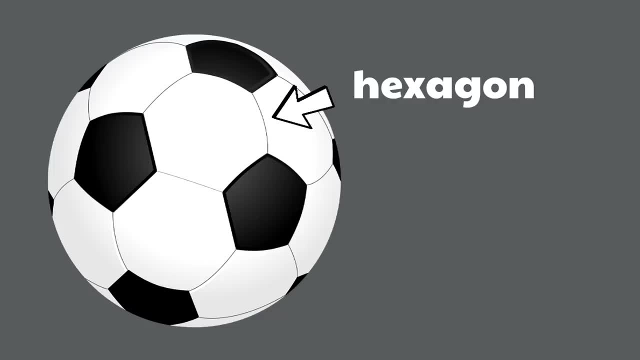 And you can see. there are six sides for each white panel on a soccer ball And each black panel is a pentagon. There are five sides for every black panel on a soccer ball. A soccer ball is covered in hexagons and pentagons. 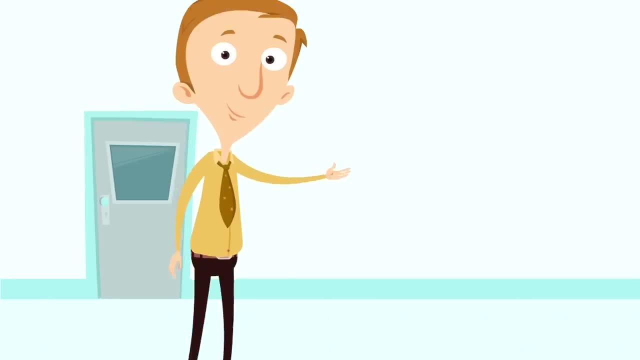 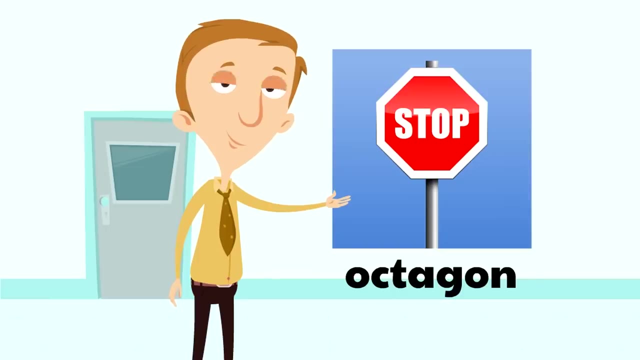 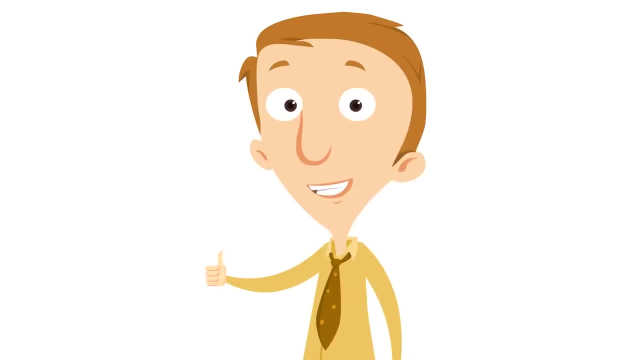 You've also seen octagons in real life. Have you ever noticed that a stop sign is an octagon? Yeah, a stop sign is an octagon. It's a shape that has eight sides. Hey, a special thumbs-up to you. 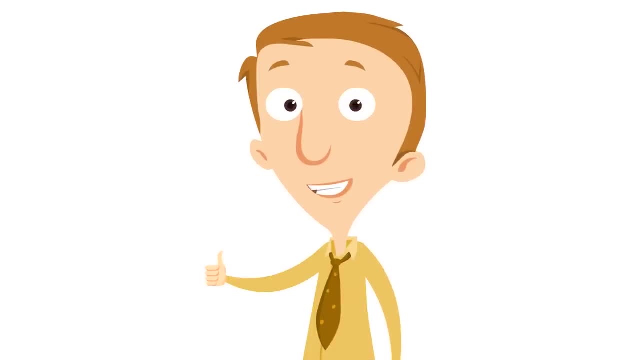 You've done a great job. In fact, you've done so well. we're gonna quiz you. Yeah, we're gonna. It's quiz time. It's quiz time. I hope you're ready. I hope you're ready. It's quiz time. 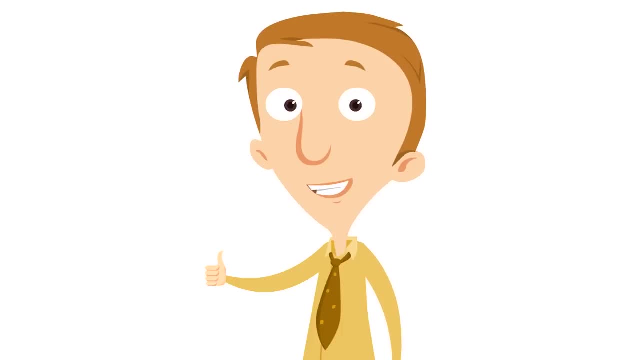 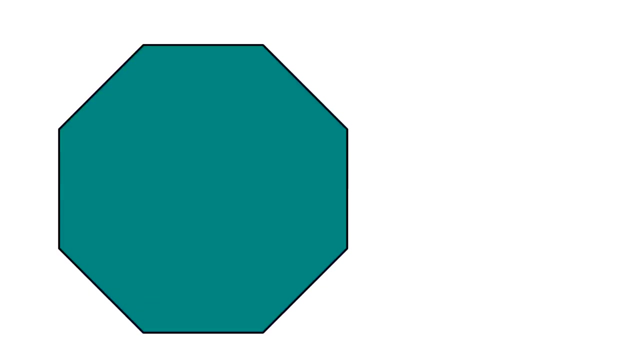 We're gonna find out how many of these shapes you can remember that. you know It's gonna be awesome. You're gonna do great. You've been paying attention. Okay, what is this shape? If you need to count the sides, go ahead. 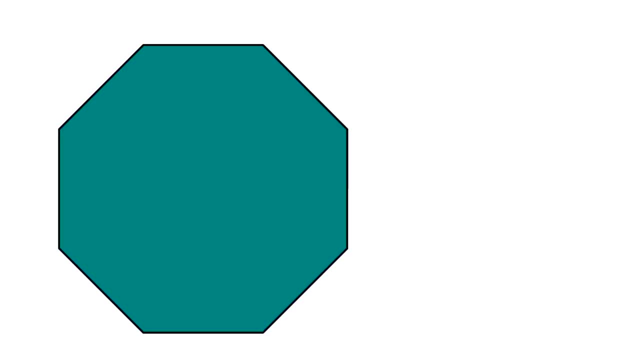 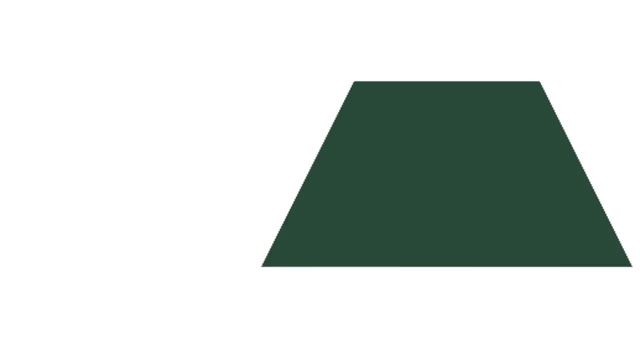 What is this shape? Uh-huh, This shape is an octagon. Good job, Okay, here's the next one. What is this shape? What is this shape? Do you remember? Uh-huh, A trapezoid. 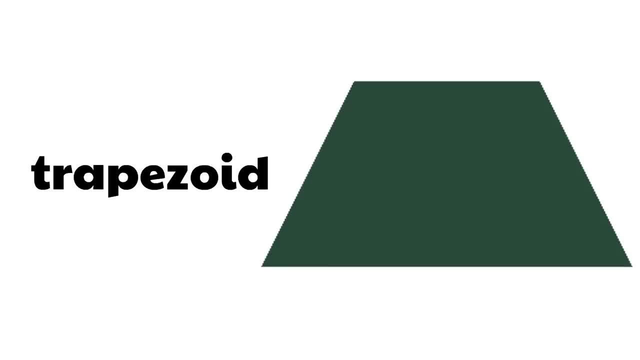 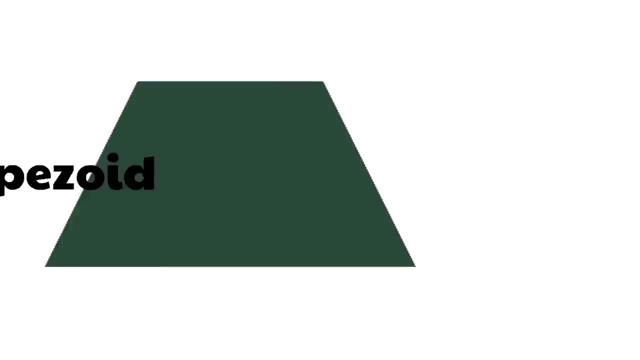 Yeah, what a fun name to say: Trapezoid. This is a trapezoid. Two of the sides are parallel to one another and the other two sides are not parallel to one another. Okay, let's try this shape. 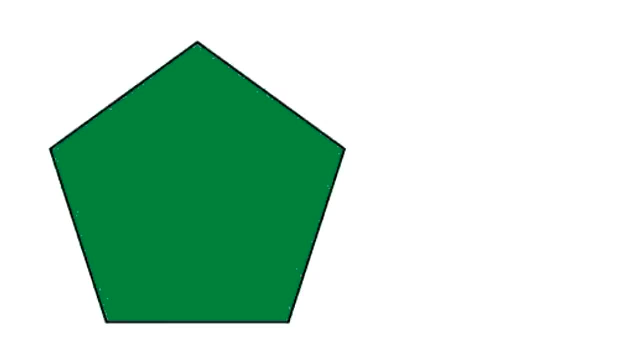 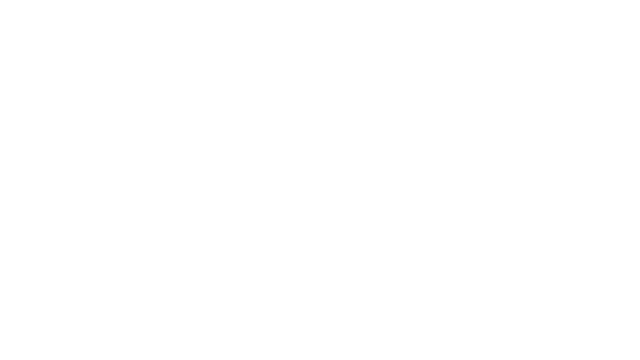 What is this shape? If you need to count up the sides, what shape is this? What shape is this? Great job, A pentagon. A pentagon has five sides. Great job. Okay, you're doing a great job. You're doing a great job. 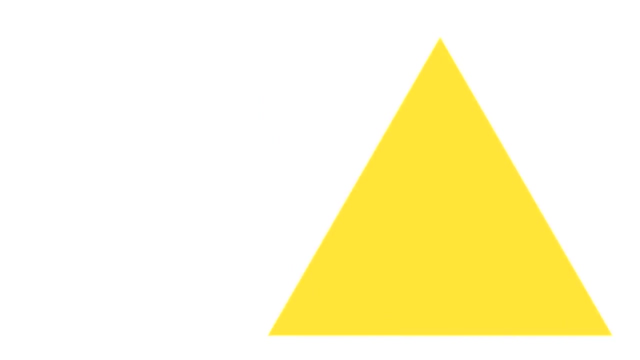 How about this shape? Okay, how about this shape? What shape is this? What shape is this? What shape is this? Yeah, a triangle, A triangle. We know it's a triangle because it has how many sides, Uh-huh, three.